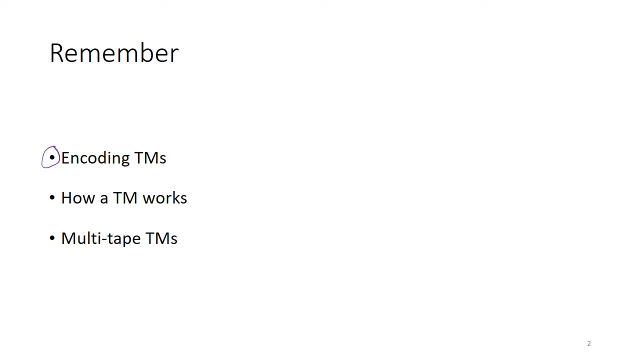 And if we can encode a Turing machine into a string, I'm going to represent that string like this: This is the encoding machine. This is the encoding of the machine M, Because we can encode all of the elements of that machine's alphabet. in our new thing, we can also encode strings that are inputs to that Turing machine. 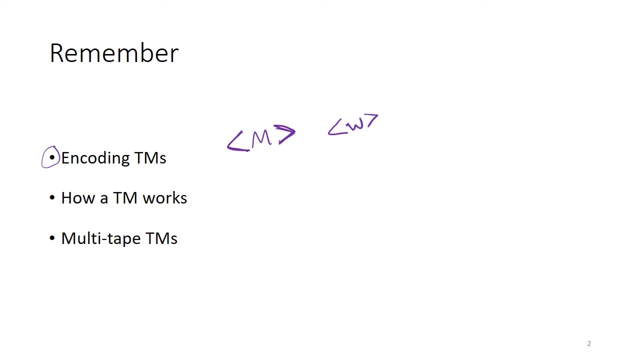 And I'm going to represent those by this. Anything in the angle brackets is now an encoded version of that. So this is the encoding of the Turing machine and this is the encoding of its input string. So when I want to talk about a machine and an input to it, 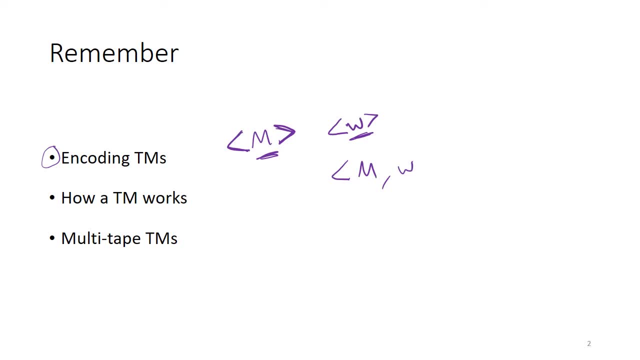 I'm going to represent it like this. So this is the pair of the encoding of the machine and the encoding of an input to that machine. What I also need you to remember is roughly how a Turing machine works, but particularly that we can have multi-tape Turing machines, and how they work. 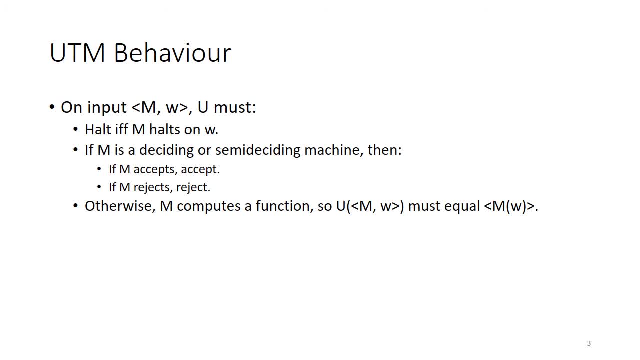 So you should have learnt that last week. So what do we want our universal Turing machine to do? So our universal Turing machine is going to be called U, And what we want it to do is accept the encoding of a machine and the encoding of an input to that machine. 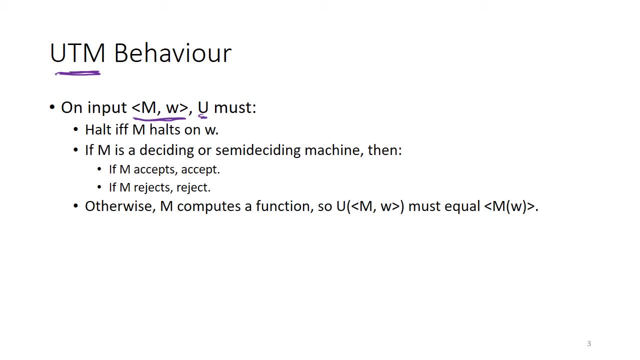 So that's what this angle brackets MW represents, And we want it to halt if and only if that machine halts on the input string. And if the machine is a deciding or semi-deciding machine, then we want the universal Turing machine that's simulating it to accept. 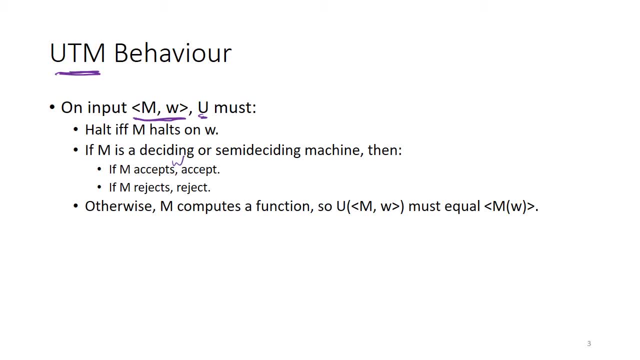 if the machine accepted W. So if M accepts W, we want our universal machine to accept this string, And if the machine rejects W, then we want this universal Turing machine to reject the encoding. If, on the other hand, our Turing machine computes a function, 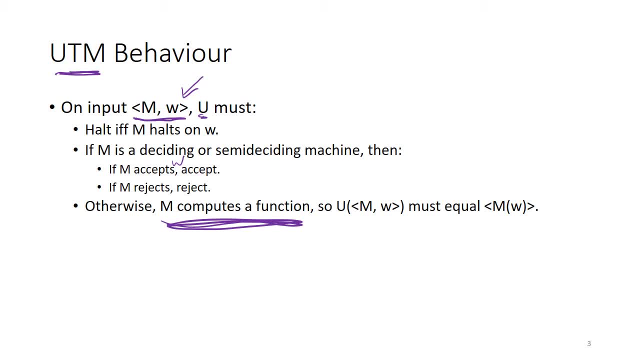 we want the output of our universal Turing machine to be the encoded result. So if our Turing machine would normally leave this value as a result, we want the universal Turing machine to leave the encoding of that value as its result when it is run on this. 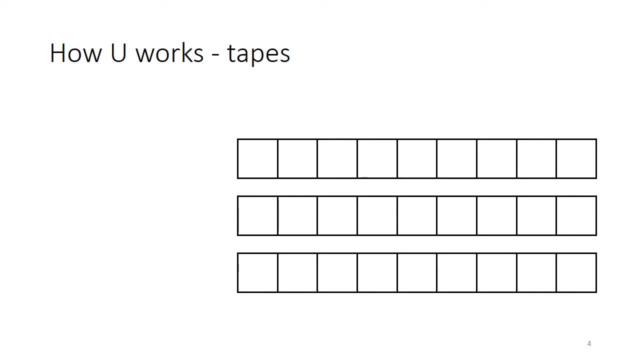 So the way our Turing machine is going to work is it's going to use three tapes. So when it starts it is going to have the encoding of the machine and the input string on the tape, on the first tape. So that's how a multi-tape Turing machine always works. 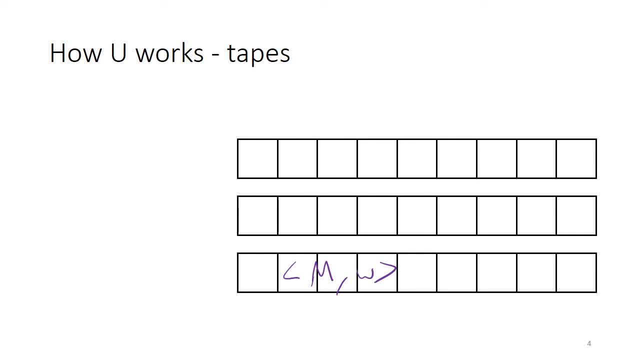 The first tape has the input and the rest of the tapes are blank. What the other two tapes are going to be used for is: this tape is going to be used as a representation of the machine. This tape is going to be used to represent the current state. 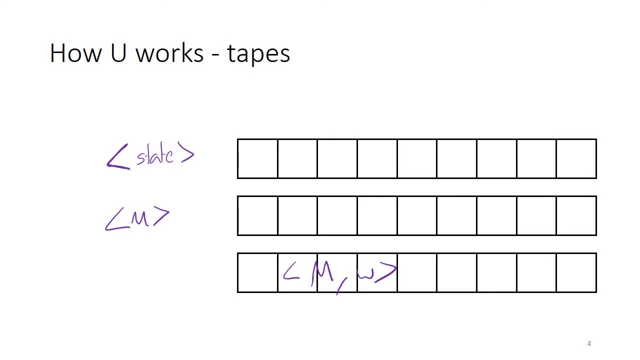 so the encoding of the current state And the original tape is going to be used as the machine's tape. So the machine itself will have a tape and that's what this bottom tape is going to be used to represent. So it's going to be the working space. 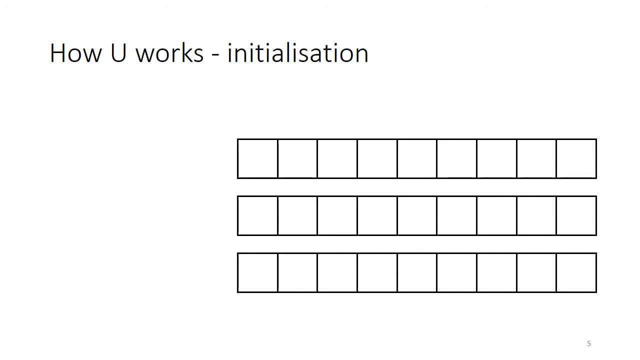 And I'll show roughly how that works down here. So the first thing our Turing machine does is it has the encoding of our machine and the input string down here, So it knows how to read Turing machine strings, and it goes through and it copies the encoding of the machine up to this tape. 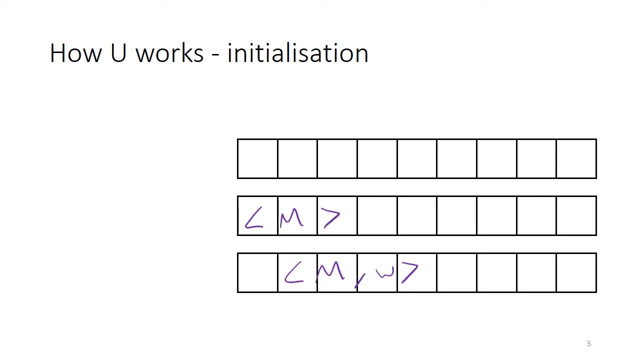 And it figures out whatever the start state is, because the start state will be the state that is labeled as 0, and it copies that onto the state tape. So this is the state tape, This is the encoding of M tape, So this tape never gets modified again. 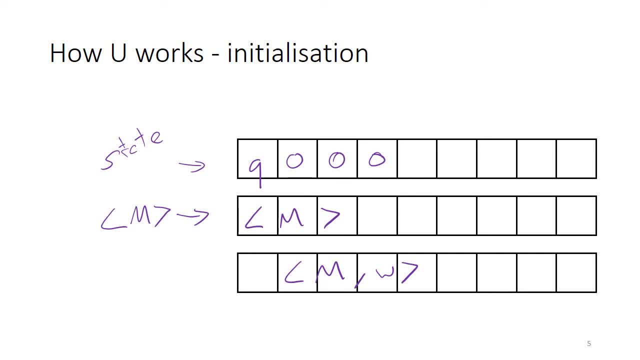 And then it leaves, finally on the bottom. it wipes everything else out and it just leaves the encoding of the input string And that's how the machine initializes itself. So it starts off with the encoding of the machine and the string. It copies the encoding of the machine off onto another tape. 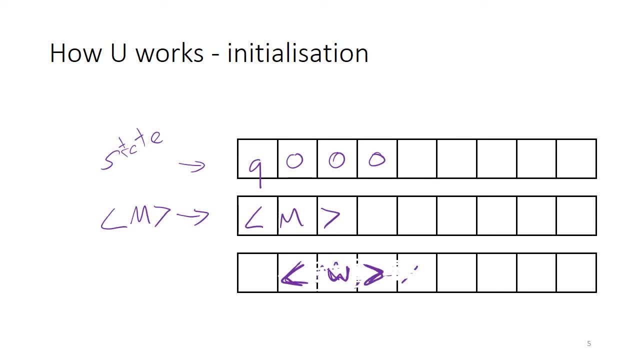 so it can look at that later. It puts the start state up on its state tape so that tape keeps track of what state it's currently in, And then it leaves the encoding of the input string on M's tape And the way the machine works is that it's going to take the input string. 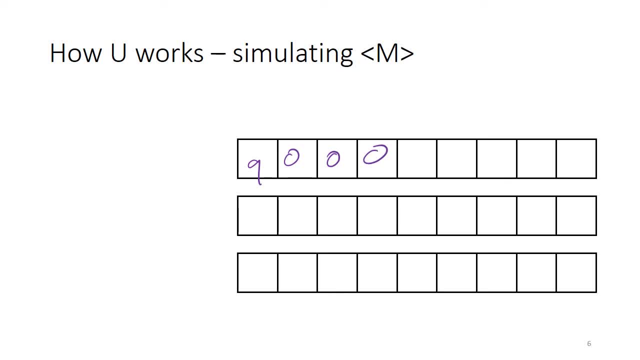 and the way the machine works from then on is very simple. So it now has the encoding of M on one tape, the current state on another tape and the encoding of the input string on the bottom state, And it simply looks at the parts that represent the first input in W.